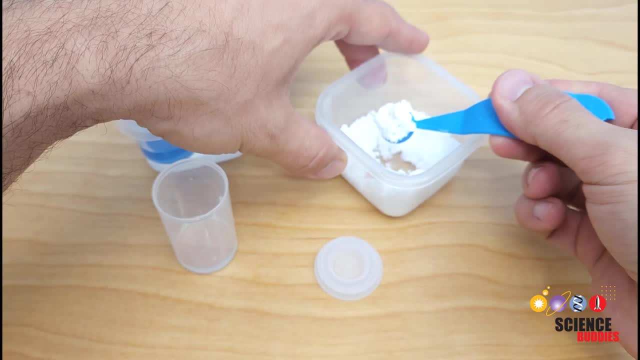 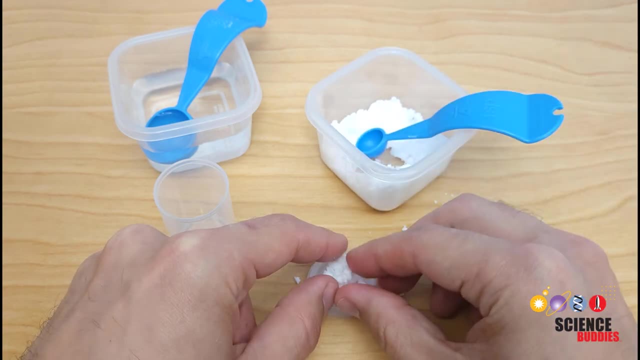 runny or too chalky. You want it to form a paste that you can scoop and pack into the lid of the film canister like this. So I'm going to take a little scoop. don't worry if you spill some. I want to be able to pack that in there tightly enough such that when I flip the lid upside down, 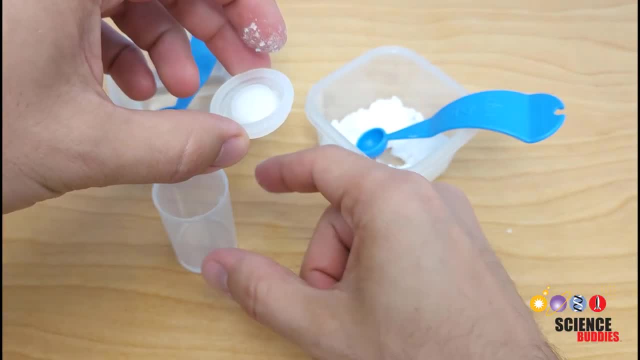 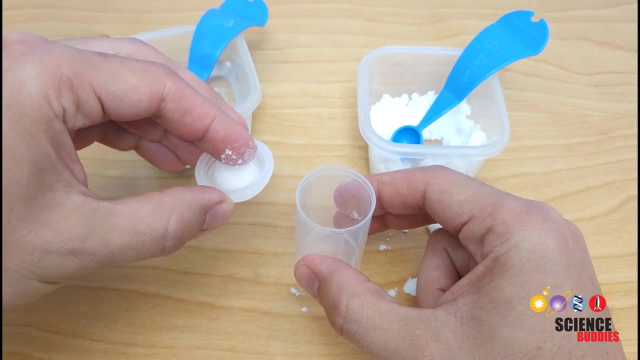 it doesn't fall out That way, and I'm not going to do this inside because I don't want the rocket to launch inside. but when I snap the lid onto the canister, the baking soda and vinegar aren't in contact yet, so the reaction doesn't start until I flip it over and the vinegar spills. 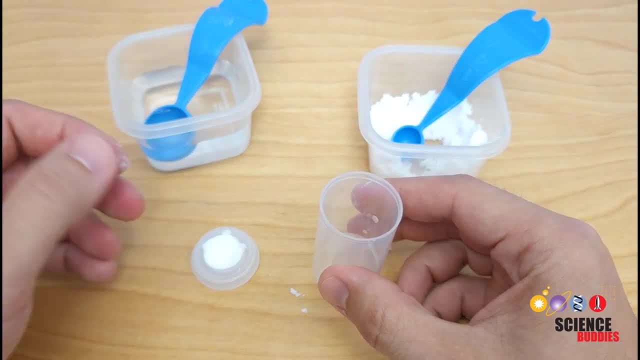 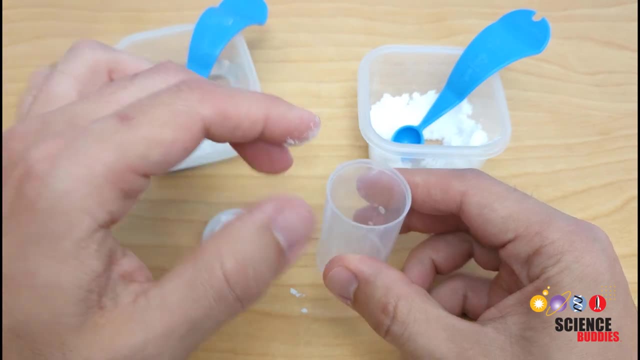 onto the baking soda, then the reaction will proceed and the rocket will launch. But that gives you a little more time. But that gives you a little more time to get things set up, as opposed to just dumping the baking soda directly into the vinegar and 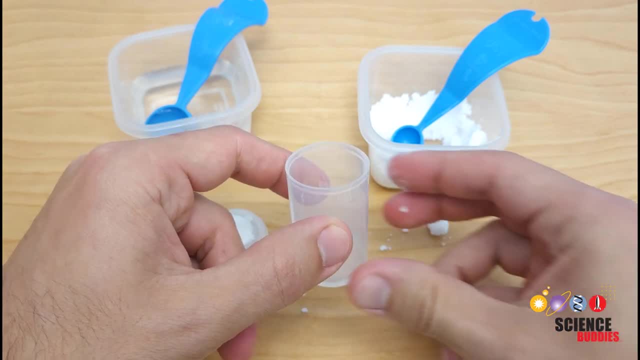 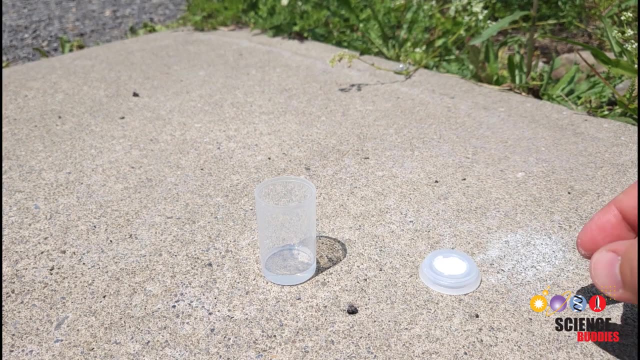 having the reaction start right away. I'm going to go try that outside, because, again, you do not want to launch these rockets inside or things are going to get a little messy. Once you're outside, again, make sure you have your safety glasses on and then gently but firmly snap the lid into place. 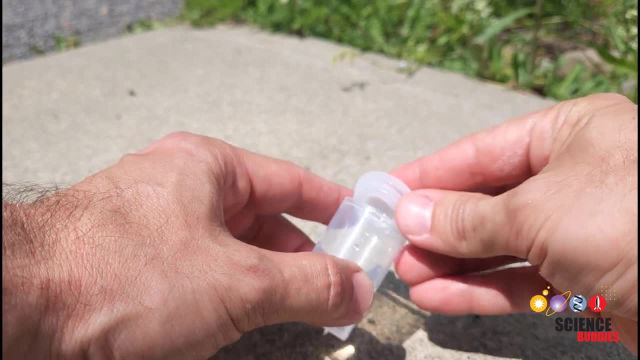 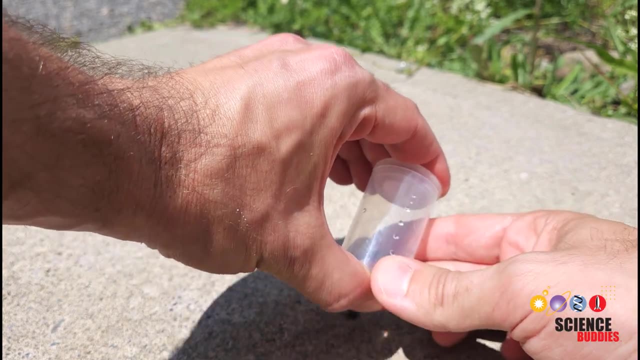 and flip the canister upside down. I say gently because you don't want to push it in so hard that you accidentally pop the baking soda out of the lid and cause it to fall into the vinegar, But you want to make sure the lid is on tight so you don't have any leaks. 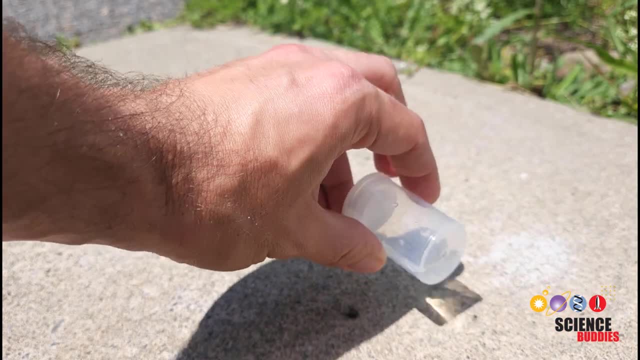 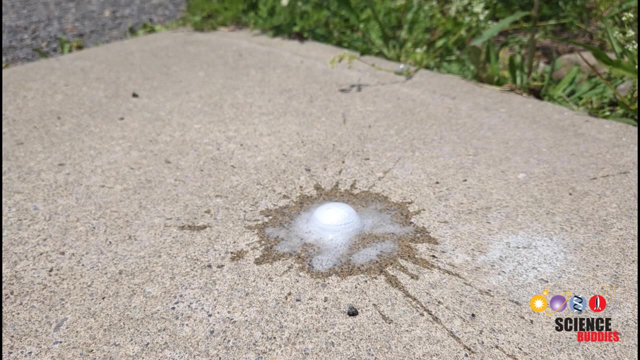 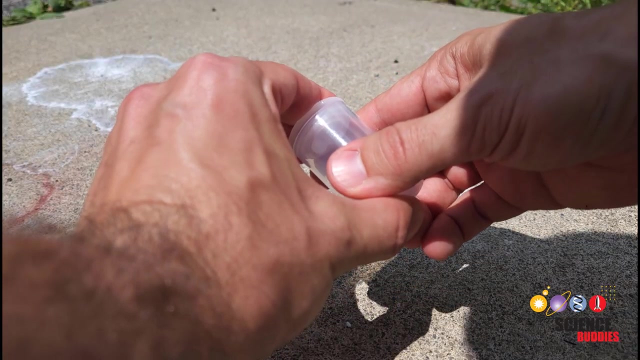 So there, I've heard the snap. I know the lid has snapped fully into place. Now I'm going to flip it over, step back and wait for the rocket to launch. Here you can see what happened when the baking soda did fall out of the lid when I snapped it on. 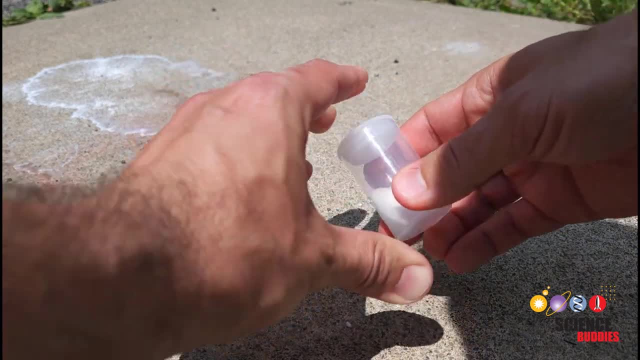 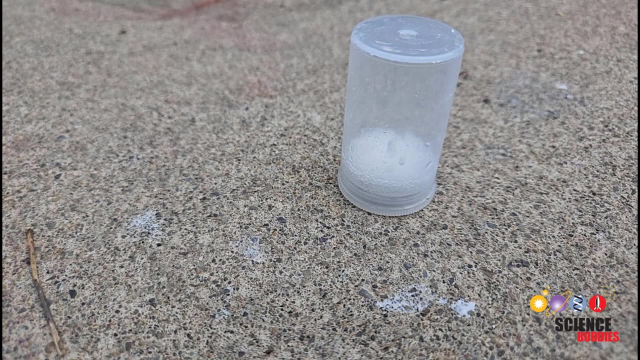 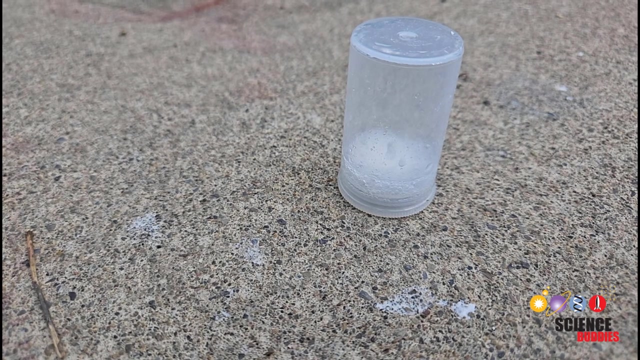 If that happens, it's okay. You just need to very quickly flip the rocket over so it doesn't go off, and then it should still launch. If we look at some close-up slow-motion video of the rocket, we can see bubbles forming inside. This is carbon dioxide gas formed by the chemical reaction. 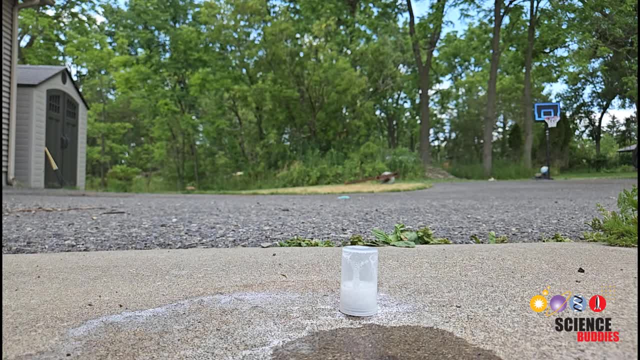 between the baking soda and the vinegar. Since the canister is sealed, this gas causes the pressure inside to build up until the lid pops off. The gas is expelled out the back of the canister at a high speed, pushing the canister up. This is why it's important to make sure the lid is on tight.